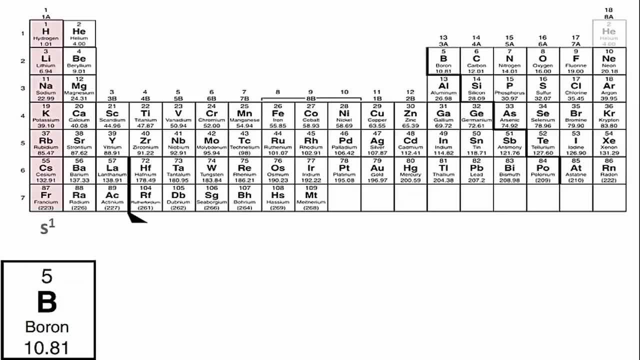 We have our periodic table and we just need to memorize that everything, every element in group 1 ends in S1.. Group 2 ends in S2.. We'll go over to the p block Those elements in group 3, they end in the p1. And then p2 all the way up to p6.. Going back to the transition, 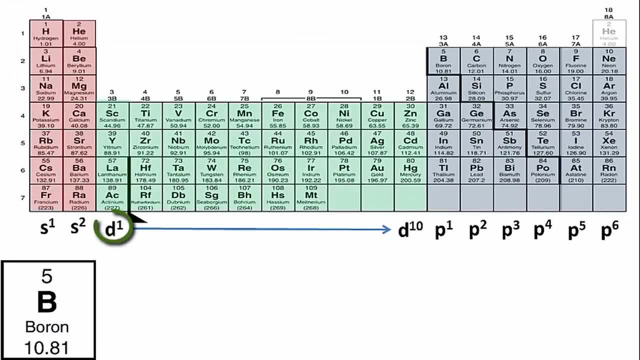 metals, we start with d, d1, and go all the way to d10.. For boron, we'll look first at rho, or period 1,. on the periodic table We can see that the hydrogen has atomic number 1, it is in rho 1, so we're going to write. 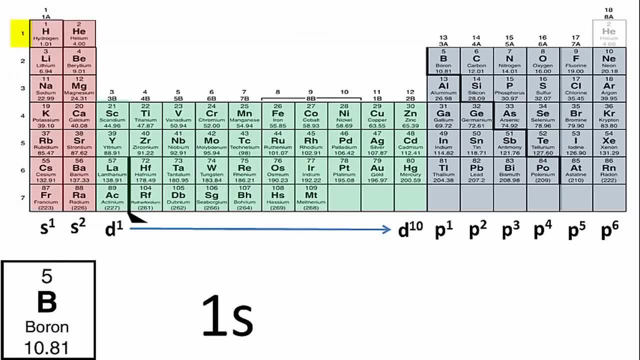 1 down. that's the period. it's also the energy level for the orbital that we're talking about. Then we'll go to number 2, which ends in s2, so we're going to call the first part 1s2,. 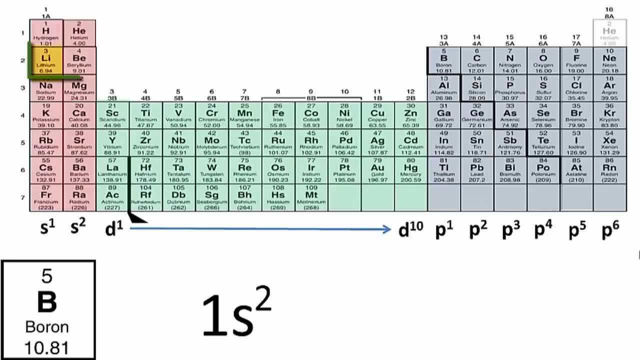 and then we're done with period 1.. We'll go to period 2, and we see that lithium, atomic number 3, that ends in s1,, next beryllium, that ends in s2, and those are all of the s's in that second period or energy level. 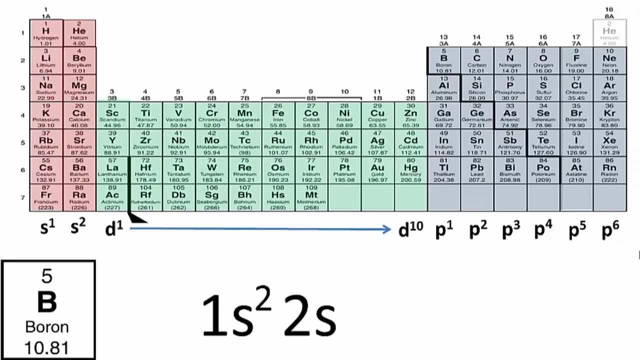 so we're going to put 2s and since there are two electrons there, 2.. Now we're going over to the p block and we're at boron, which is the element we're writing the configuration for, and we can see that boron ends in p1. 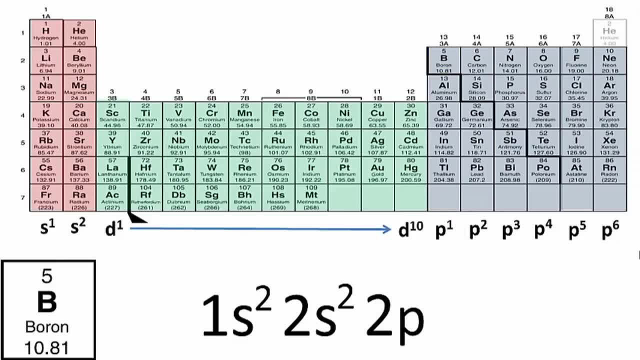 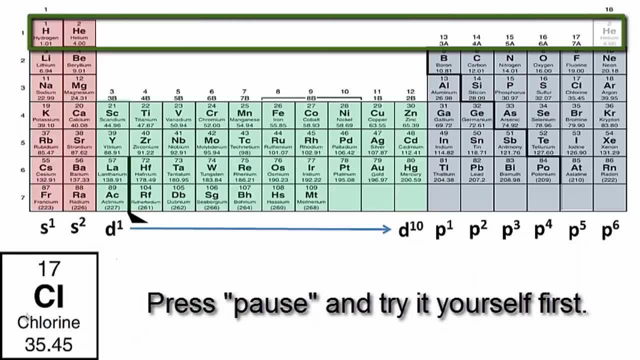 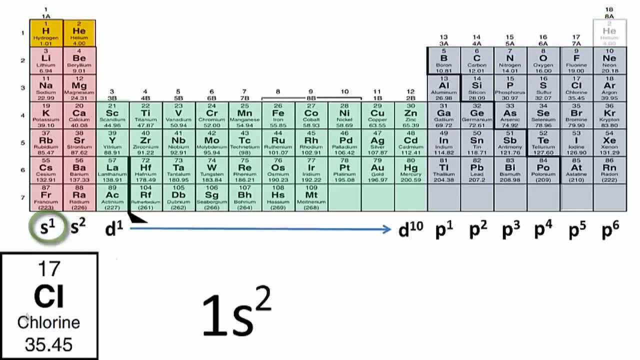 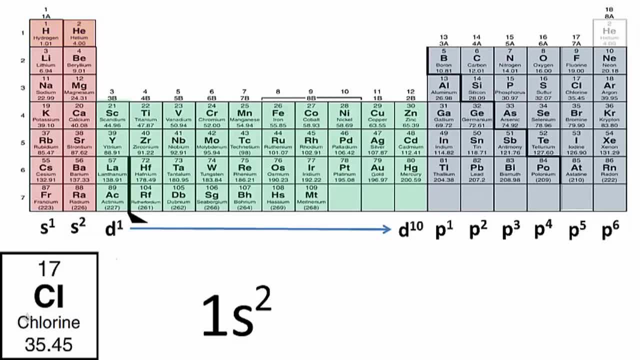 we'll start atomic number 1, we have the 1s1 and 1s2 full, so we just write 1s2, we go across and we're actually back in row or period 2, so we have lithium and beryllium, 2s2, that's. 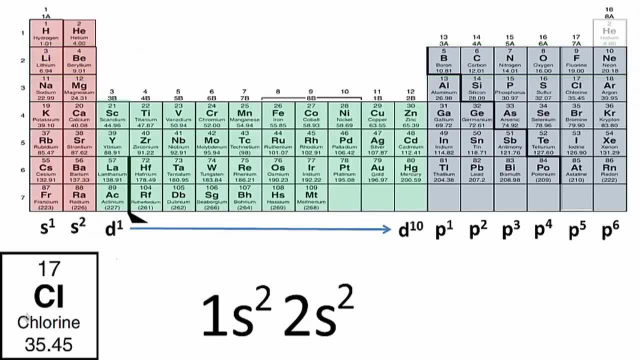 full over to the p block and we have all of that full p1 through p6, so we just need to write 2p6. we go down to row three. we have 3s1 and 3s2. those are full, so we. 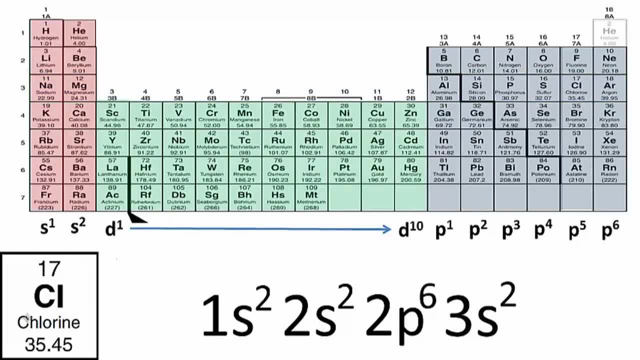 write 3s2, we're back over across to the p block and we can see chlorines there at p5. so we're almost there. so we put 3p and since chlorines in the p5 group, 3p5- that's the electron configuration for chlorine- we'll try one more vanadium. 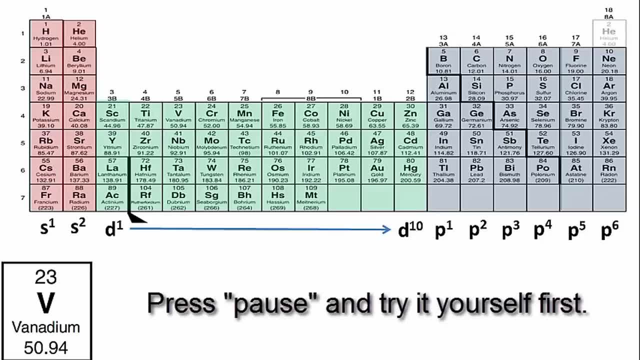 so vanadium has atomic number 23. so we have 23 electrons and we're going to go through the periodic table until we get the vanadium. so we'll start in period 1 there with hydrogen atomic number 1 and we see the 1s1 and 1s2. those are full. so 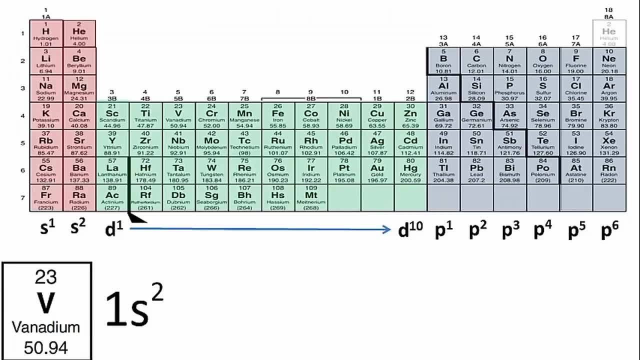 we'll write 1s2. now we move down to the second period. we have the 2s1 and 2s2 and we're back over across to row three. we have 2s1 and 2s2. those are full, so we'll write 2s2. now we move down to the second period. we have the 2s1 and 2s2. 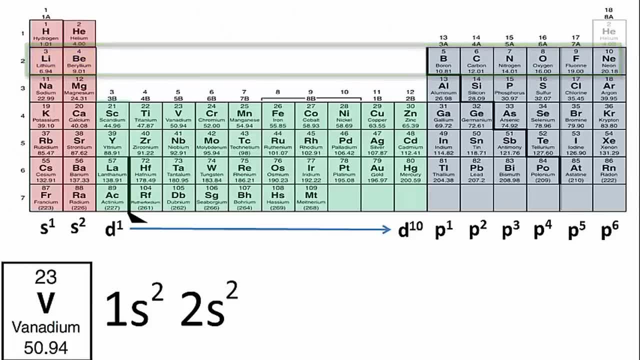 2.. Those are full. Then we go across, We're into the 2p's and all of the p's are full. So we'll put 2p 6, down to period 3,, 3s, 2.. Then we have all of the 3p's. Those are. 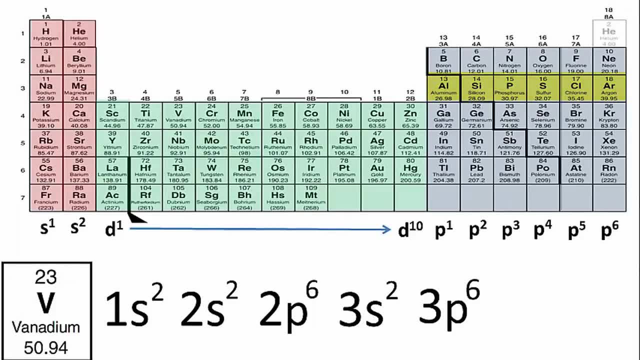 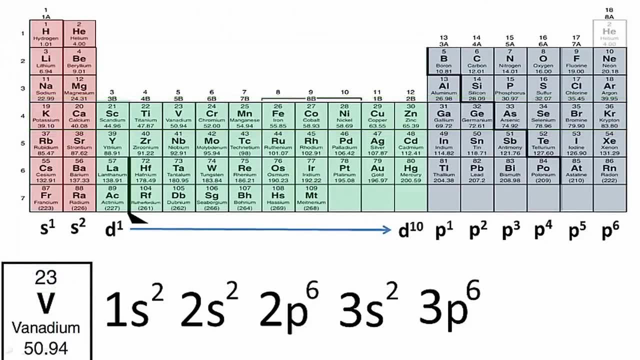 full as well, So 3p 6. We're down to period 4 and we're getting close to those 23 electrons that we have for vanadium. So in period 4, we have 4s 1 and 4s 2.. Those are full, so 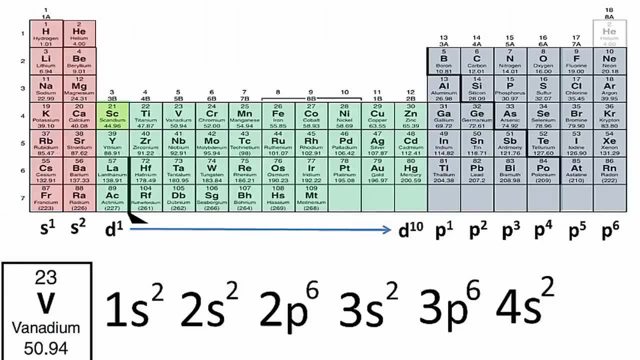 we'll write 4s 2.. And then we're into that d block there, and if we go over 1,, 2,, 3, that's where vanadium is. So we would expect that we would have 4d 3.. However, this is the. 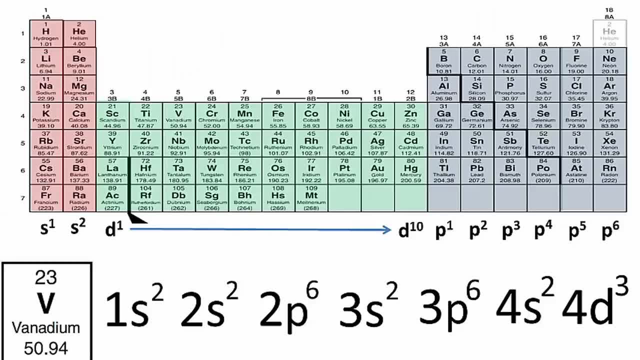 one exception that you need to be aware of if you're using this method: When we get to the d block, we always take one away from the d block, From the period number. So instead of 4d 3, we would have 3d 3 as the electron configuration.